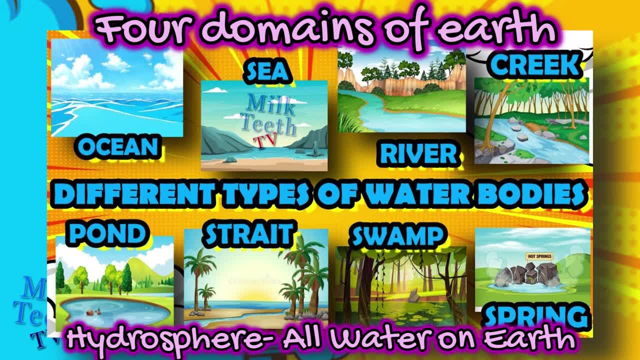 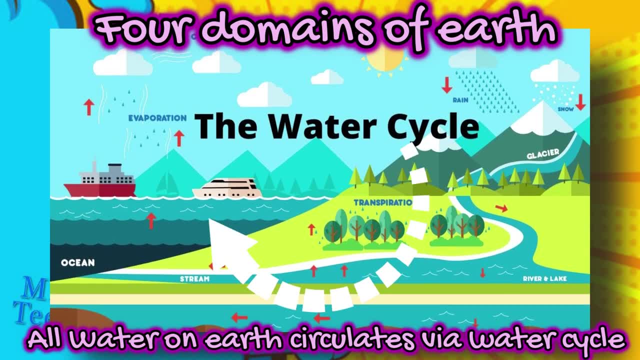 the hydrosphere. All water on earth undergoes a continuous cycle known as the water cycle, The water cyclethere is a continous cycle called the water cycle. The water cycle is also an important part of the hydrosphere, the domain of water on earth. There are some information related to the water cycle that we use on earth. All Jearnies with water, Charlotte and Emily. Apparently, there's no water lacquer or particular soil noticed on earth. there is only water in this valley. This name has been given in many different areas of each country성. 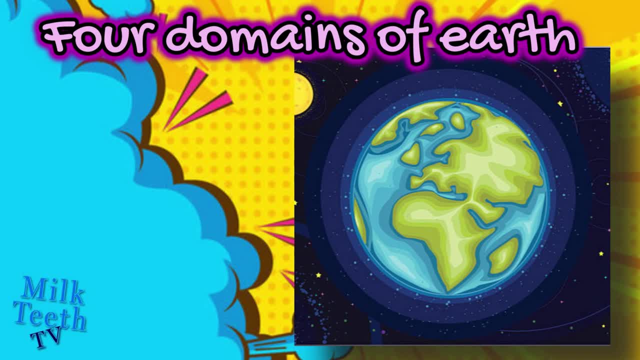 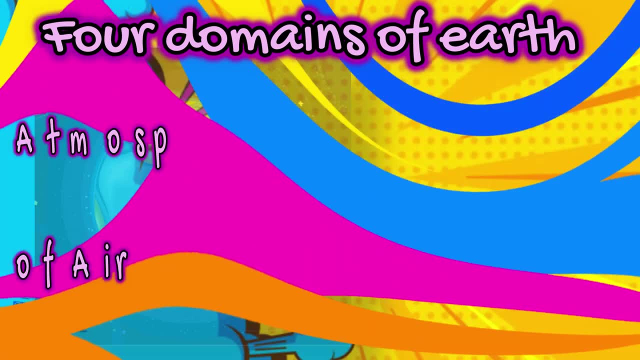 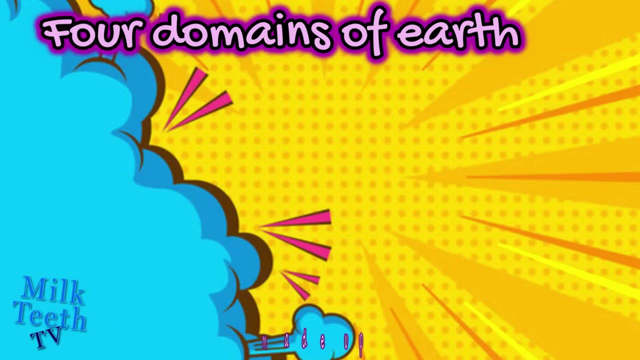 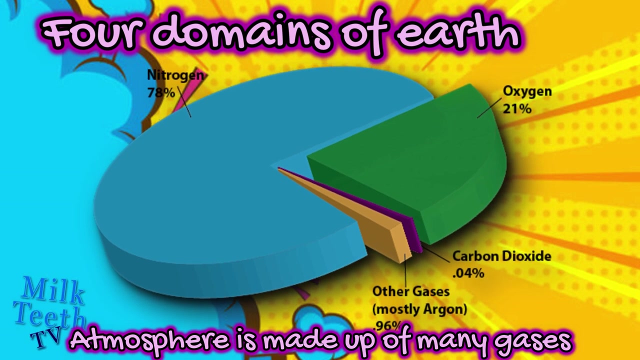 We find the water Introductionadioconamiac to the third domain of earth, which is the atmosphere. The atmosphere is the domain of air on earth. The air around us and our planet is called atmosphere. The atmosphere on earth is made up of several gases. The atmosphere of the earth is made up of about 78% nitrogen gas. 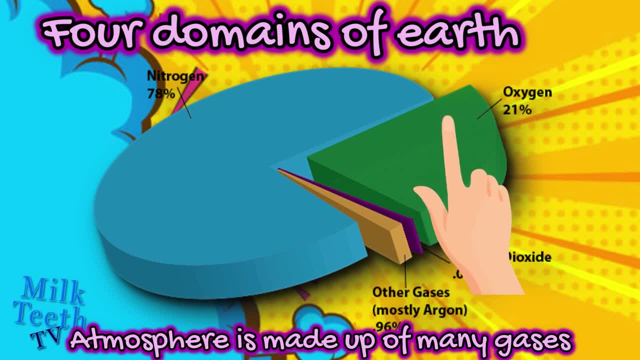 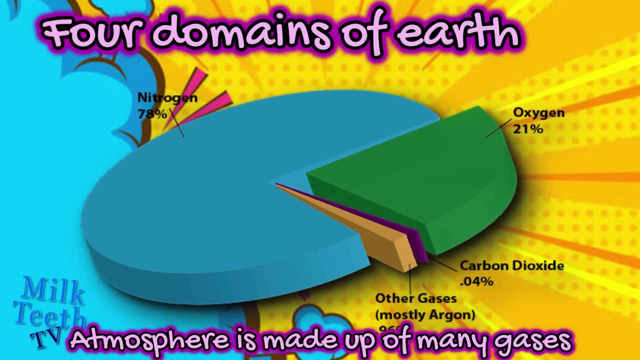 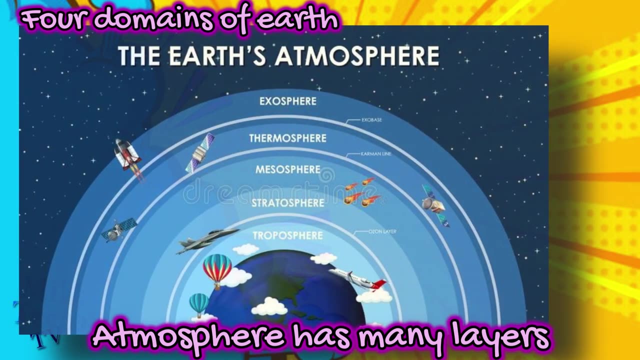 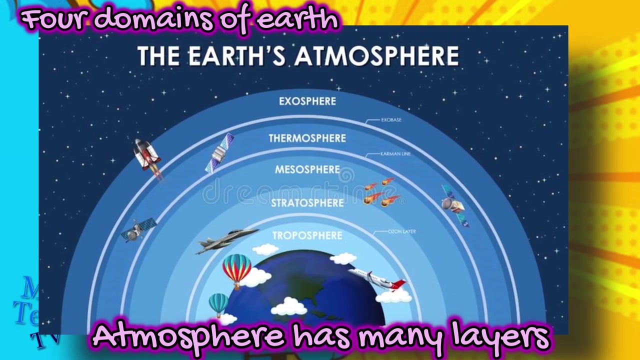 21% of oxygen gas that all the living beings breathe, and 1% of other gases like carbon dioxide and mostly argon. The atmosphere also has several layers. Layers are namely the troposphere, which is the lowest layer, which starts from the ground level and extends up to 10 kilometers. We humans 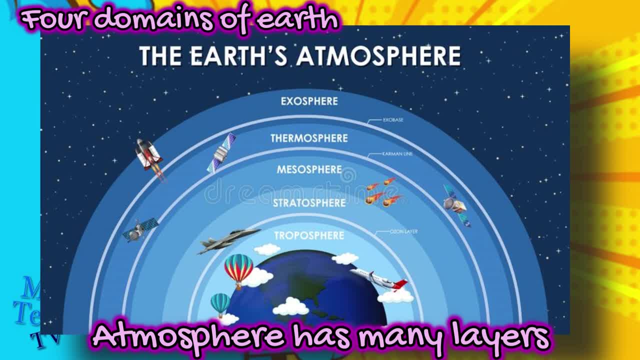 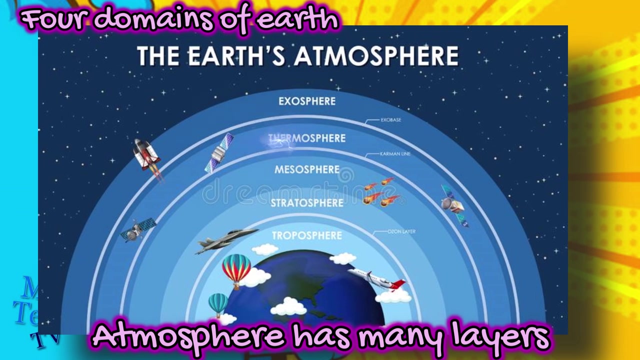 live in this layer. Next comes the stratosphere. The ozone layer is found within the stratosphere and it absorbs high energy ultraviolet light from the sun. Next comes the mesosphere. Most of the meteors burn up in the mesosphere. Then we have the thermosphere. High energy X-rays and UV radiation from the sun are 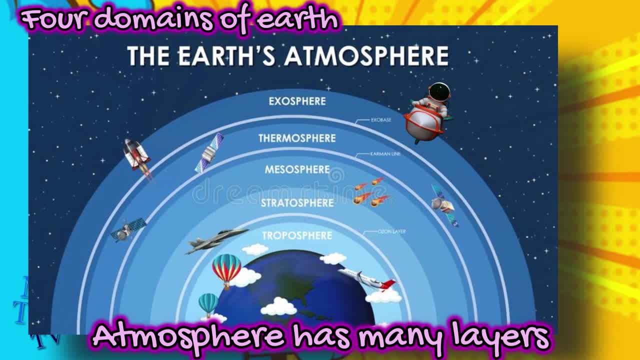 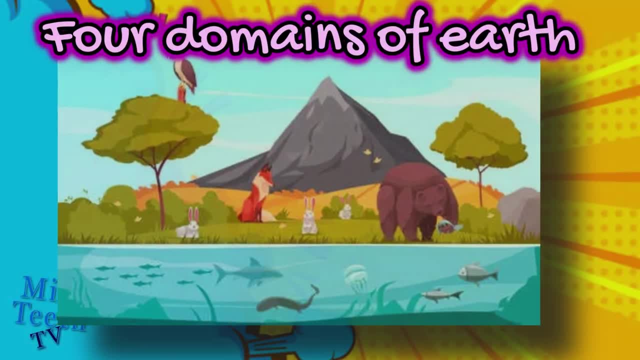 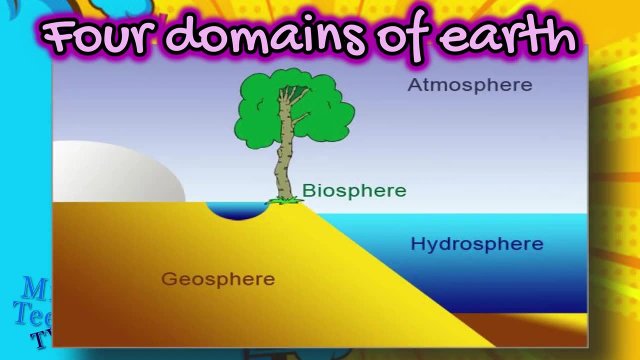 absorbed in the thermosphere. Lastly, we have the exosphere, which is the outermost layer of the atmosphere. The most important and unique domain is called the biosphere. What is the biosphere? Biosphere is the domain of life on earth. The biosphere is the zone where the lithosphere